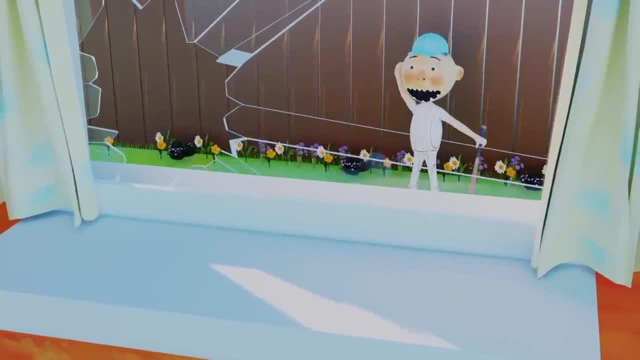 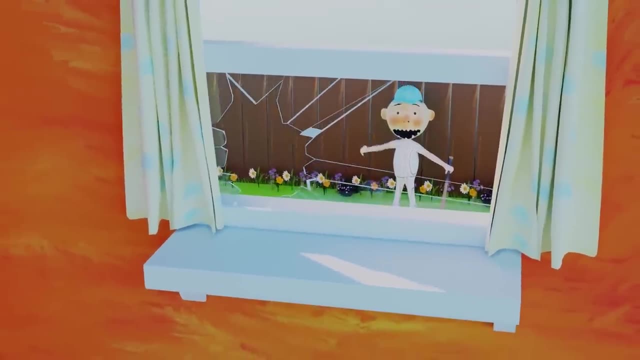 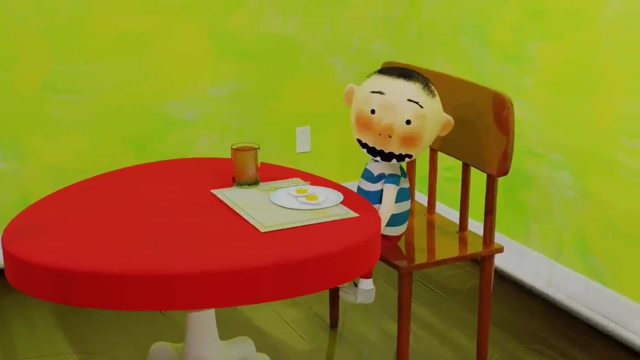 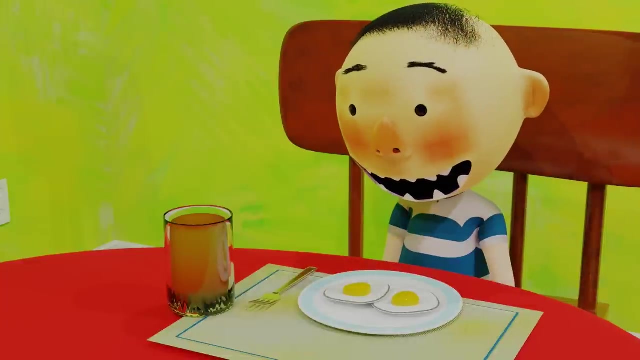 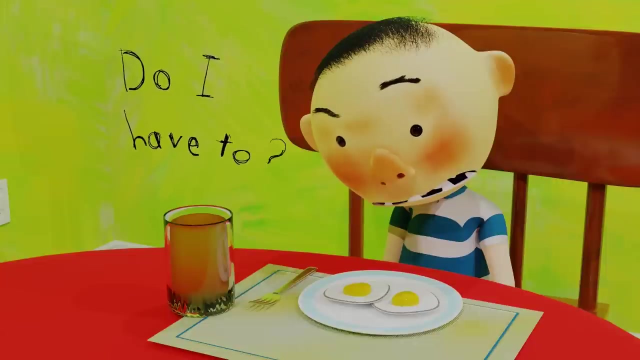 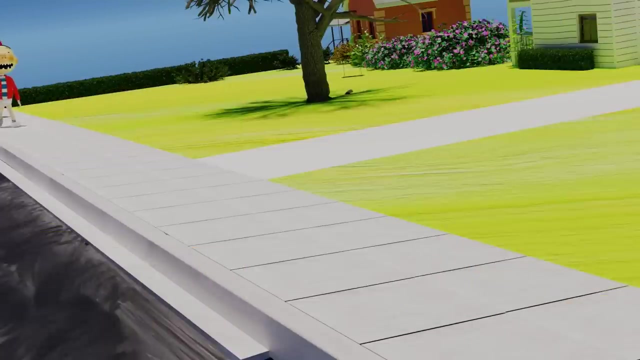 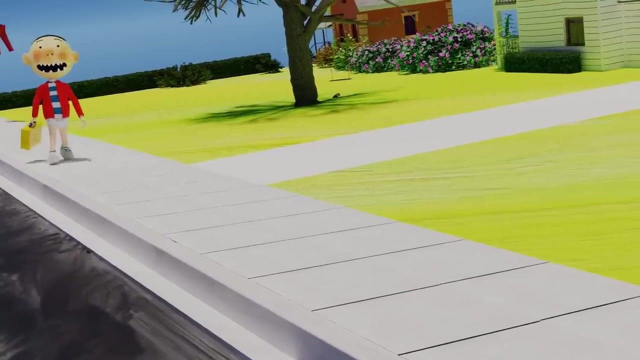 broke the glass. he was an accident. gosh cartoon. he's watching the pathway. some eggs for breakfast and juice, yummy, you like your breakfast. you go to eat. do I have to wait, David? wait, is that my imagination? or David's got no pants on? where are your? 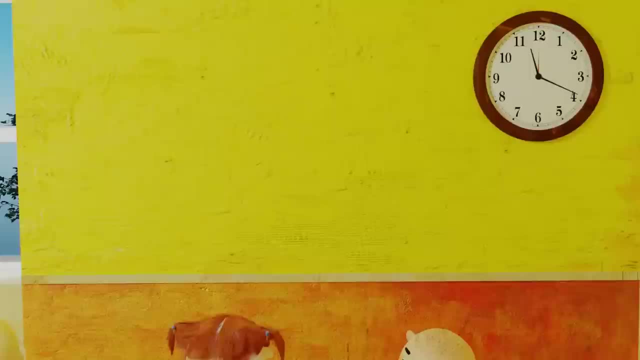 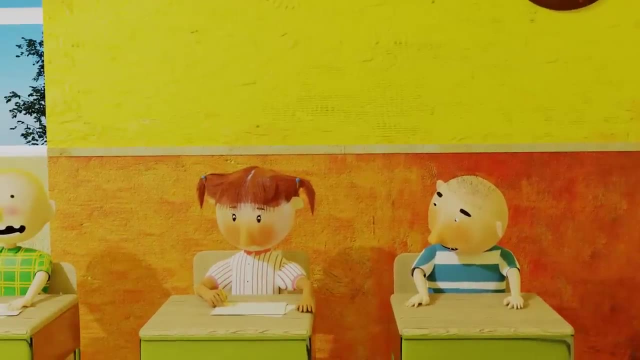 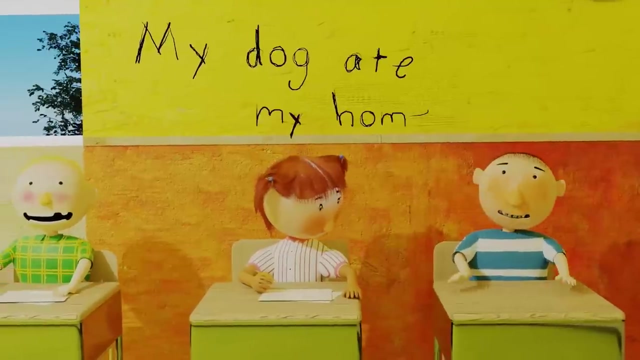 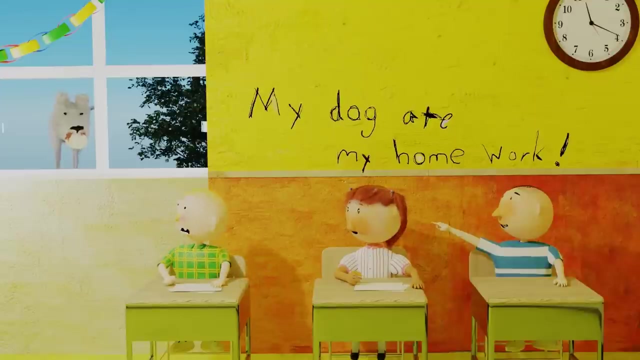 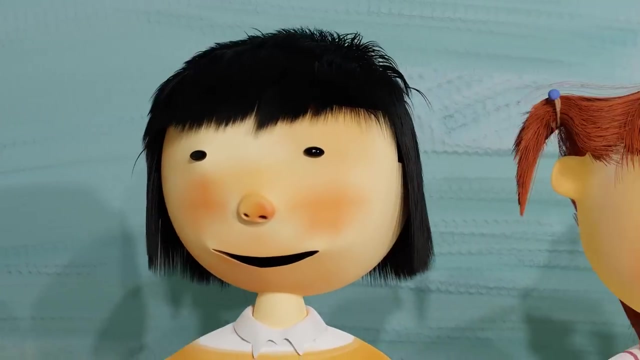 pants. oh, school time. hey, David, where's your homework? did you do your homework, my dog? I mean, your friends can't blame you, but I do look at that puppy behind a window. it's got something in his mouth. Oh, your dog ate my homework. Oh, I can tell that they are preparing for a school picture, Am I right? 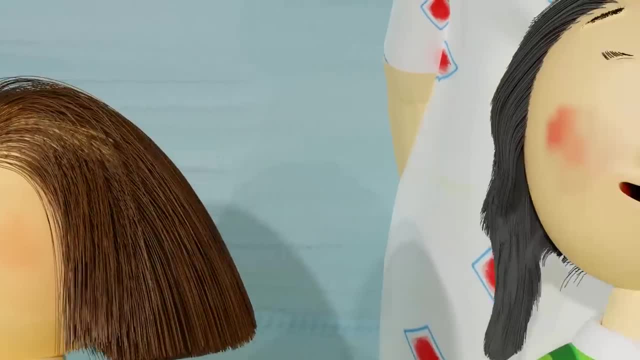 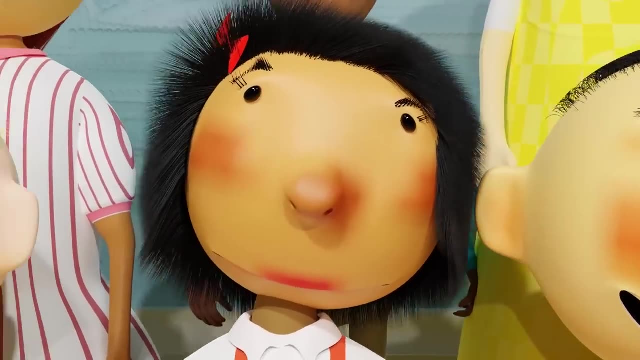 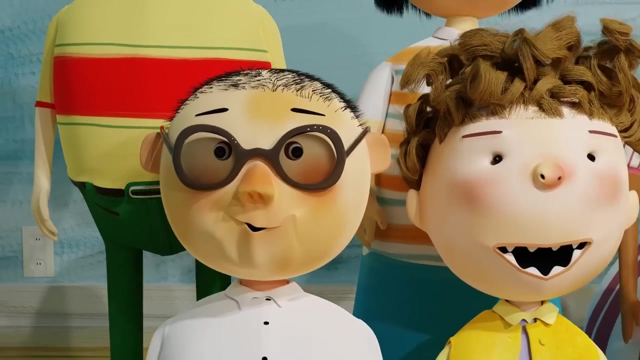 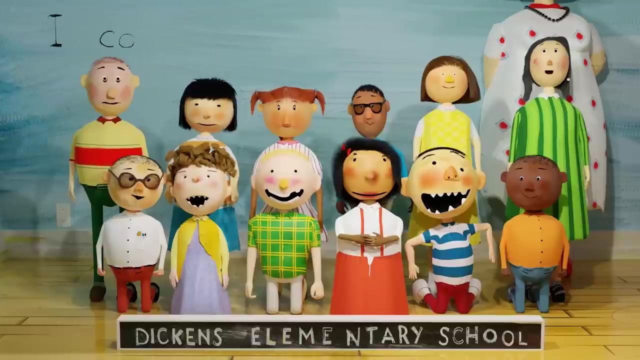 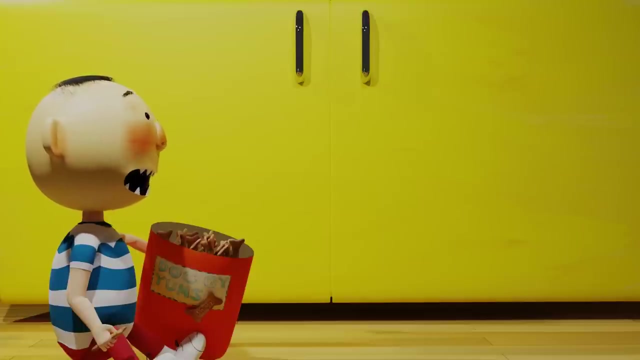 everybody standing. they find his clothes and cameraman is asking: hey, everybody smile and say cheese and Three, two, one. Oh no, you ruined a school picture, David. What are you doing? I couldn't help it. Are you eating dog food? That's disgusting. 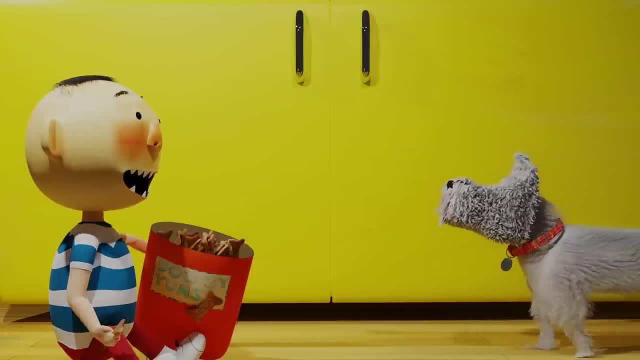 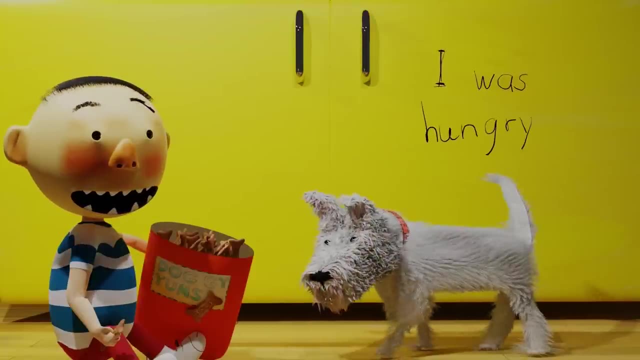 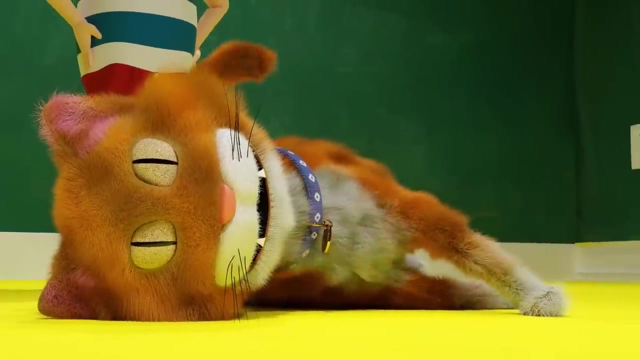 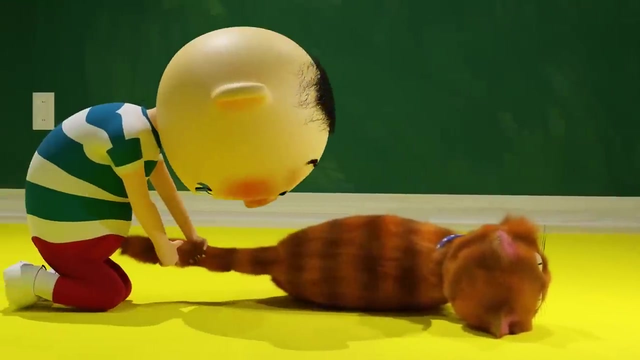 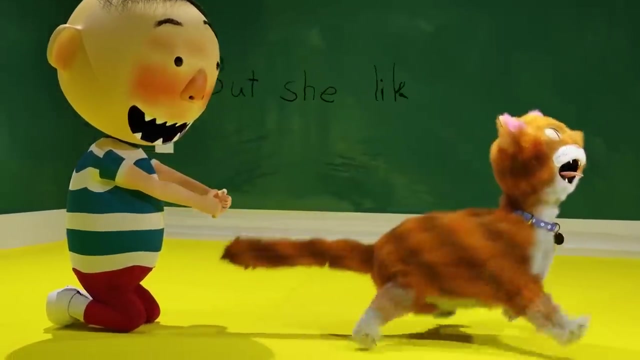 You're gonna end up in a tail. Why? you got cute pet? look at that cat, beautiful. Uh-oh, you got a wrong idea. You don't want to touch your tail. Oh no, Cats don't like it When you touch their tail, But she likes it. 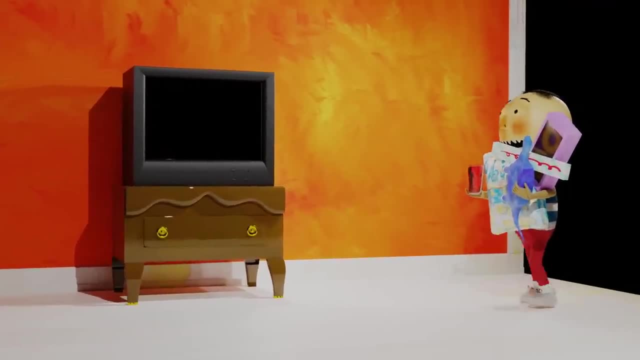 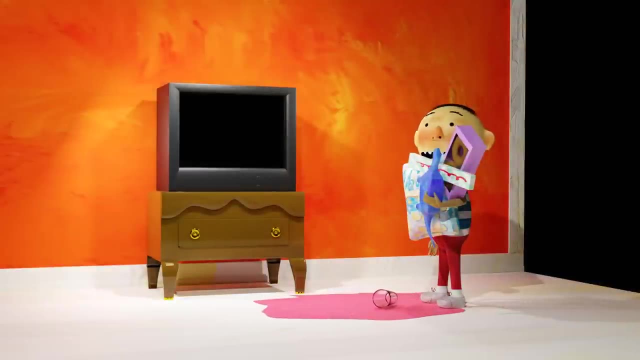 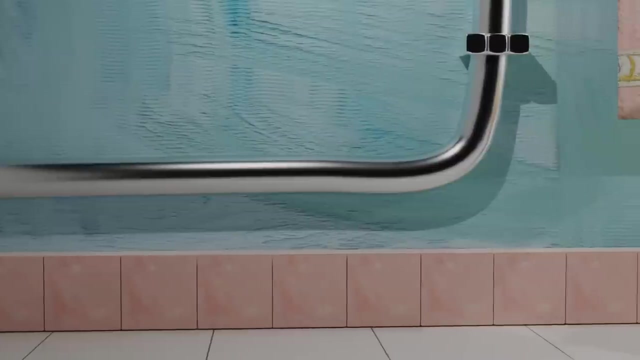 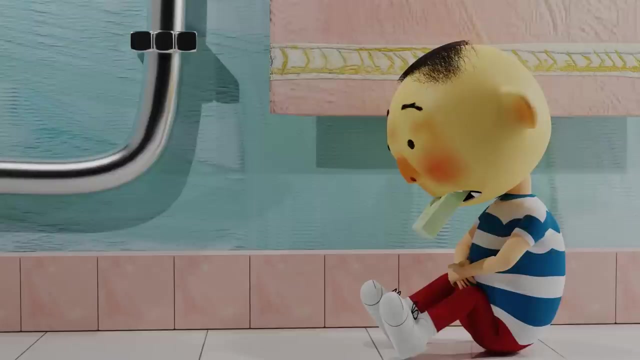 Are you carrying lots of things: some doughnuts, a Twizzler rope, a diner and bag of juice. Oh, what did you? drop a glass of juice on a carpet, Uh-oh, But it slipped a Bar of soap in your mouth. take it out. But that says it, I see, because you said a bad word, not good. 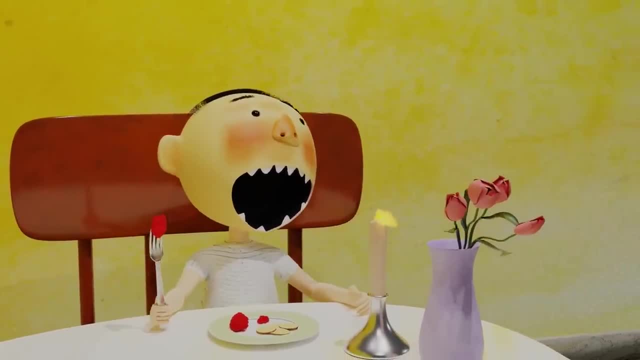 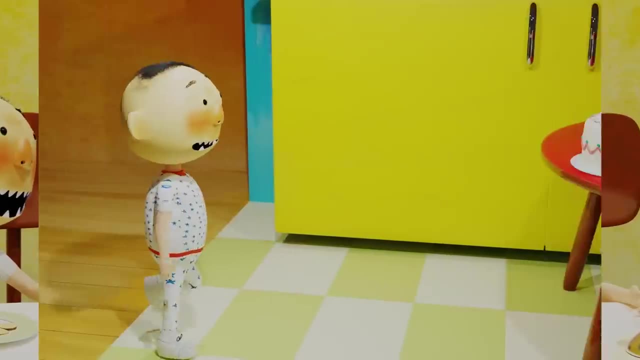 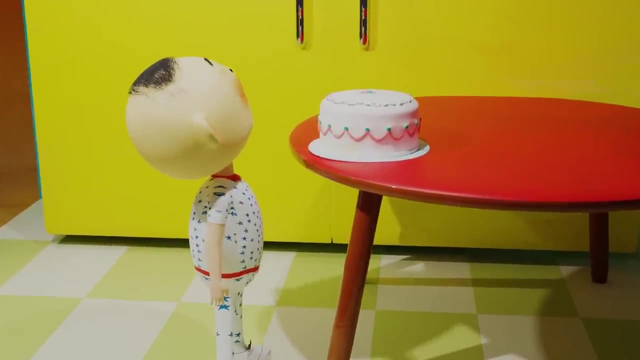 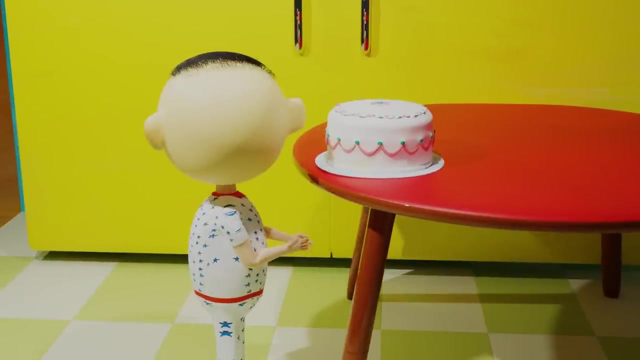 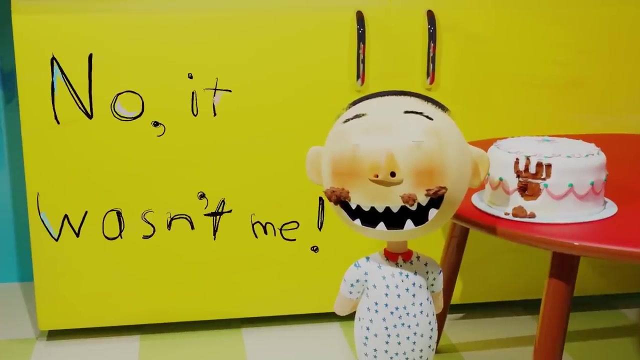 Whoa, No burping at a table. Excuse me, Nice cake. You're not gonna touch that cake, all right, No touching. no, I can see you. Did you touch that cake? no, it wasn't me. Uh-huh, Your mommy's gonna send you to bed. 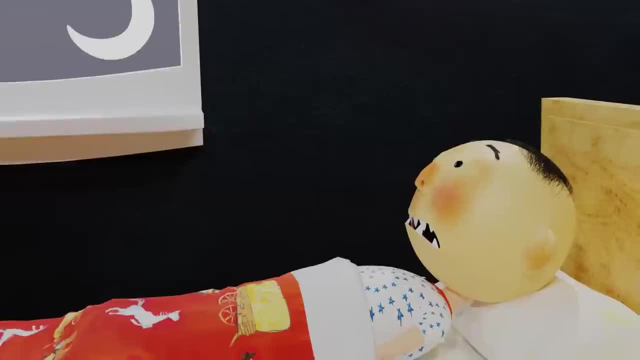 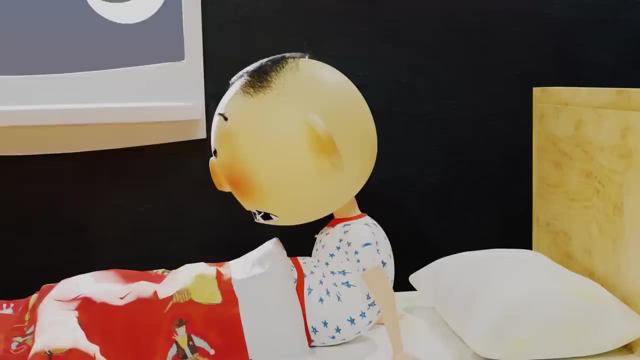 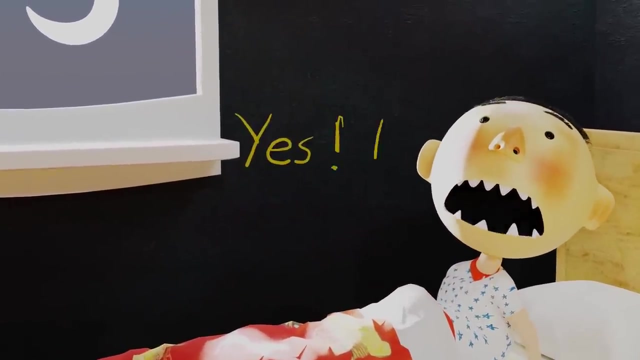 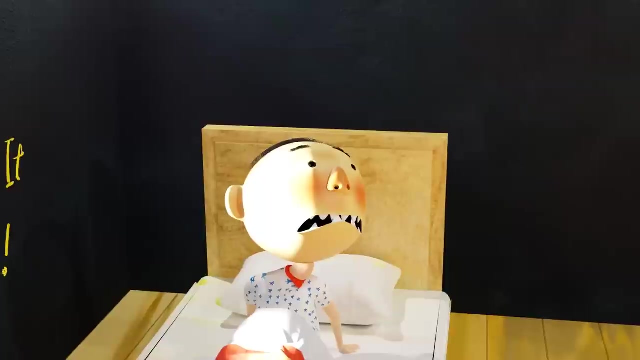 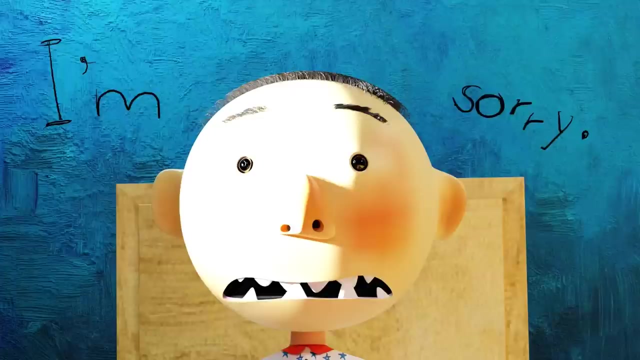 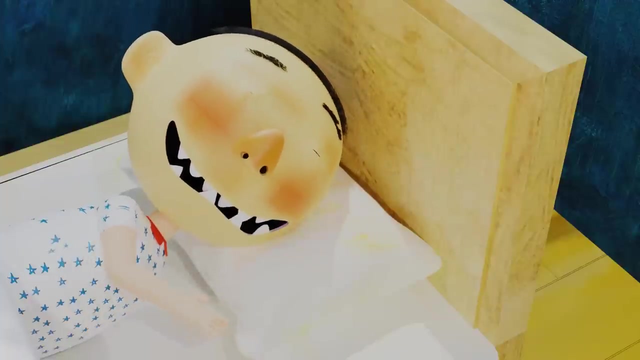 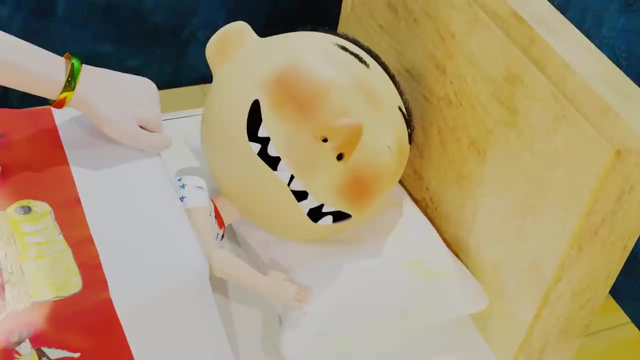 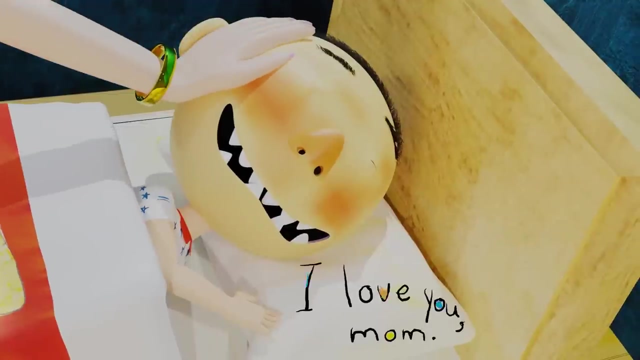 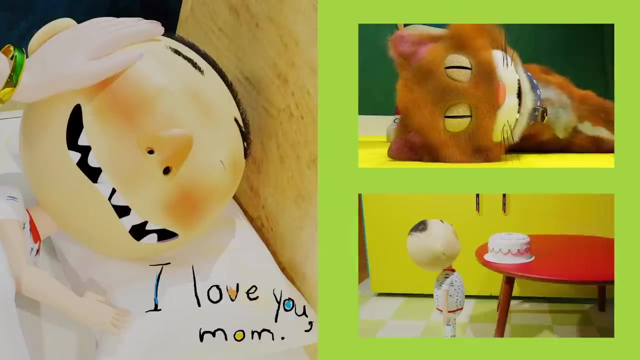 Yeah, eventually knew it. You guys come in. Did you touch that cake, David? yes, he was me. I, I, I, Mm-hmm. What's the matter with you, mom? I'm sorry. I'm sorry, hey, David, if you make any mistakes, you apologize in the first place and it'll be gone unpunished. 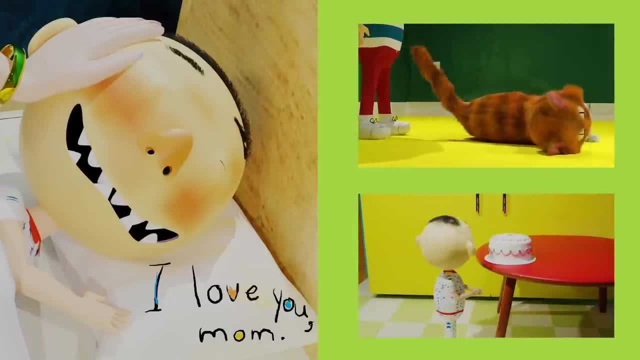 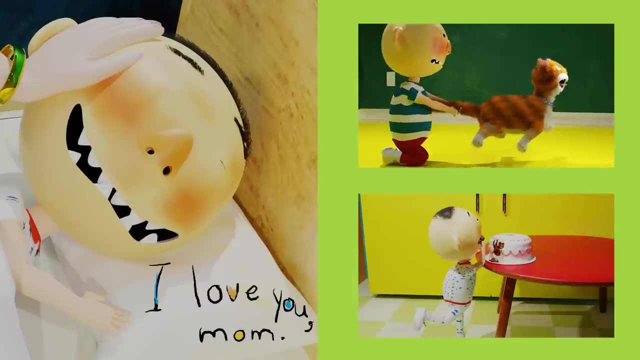 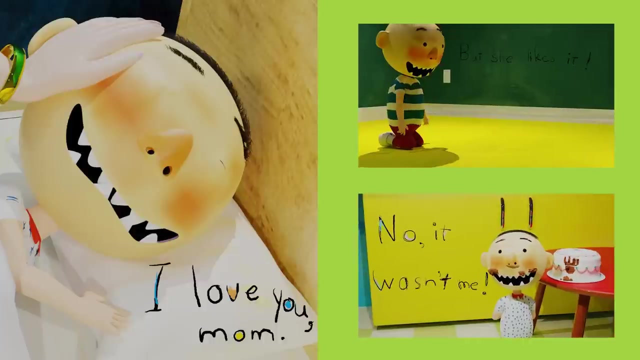 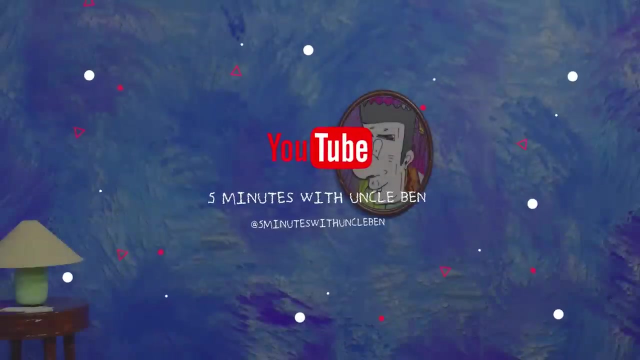 or be forgotten, and it'll be rewarded some places. so don't tell a lie, because by telling a lie you make the second mistake. so just tell the truth. all right, hope you enjoyed this beautiful story by David Shannon. please drop likes and if you want to get notified by upcoming videos, or let's say,